Sometimes organizations refuse to be part of the province. Sometimes there's not enough money and other sector agents are required to provide diye votions to pay state and state insurance writers. As a result, families are in the middle of nowhere. Human rights מת. 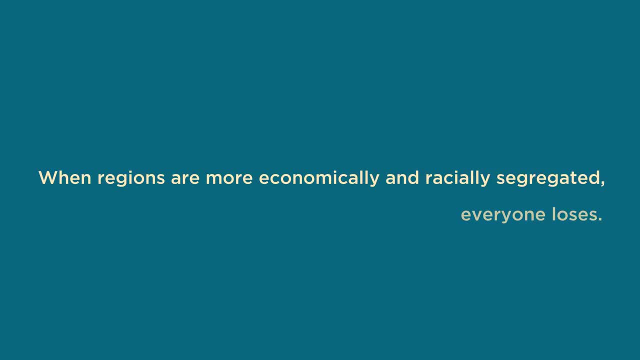 the initial phase by promulgating based social- хотяally bad- gender issue. затmok tripauti making housing donor centers said they had it's only one state urgent that their and racially segregated everyone loses. Local economies see slower growth and. 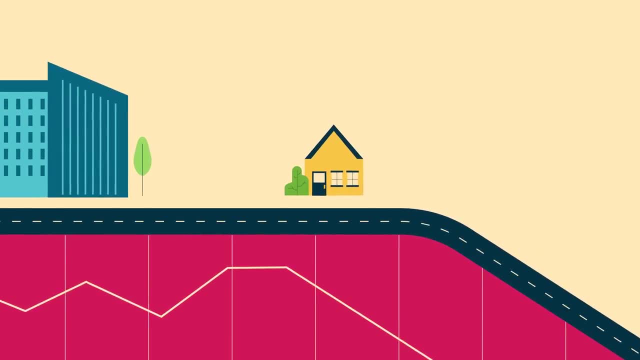 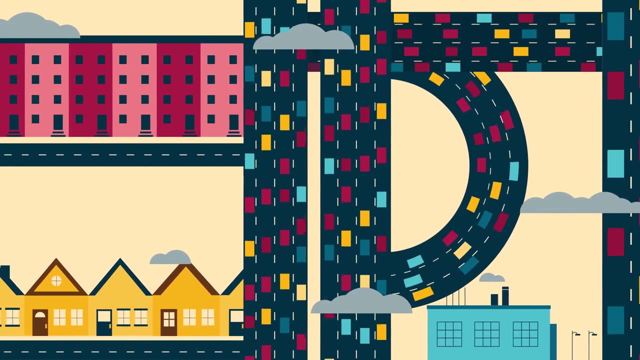 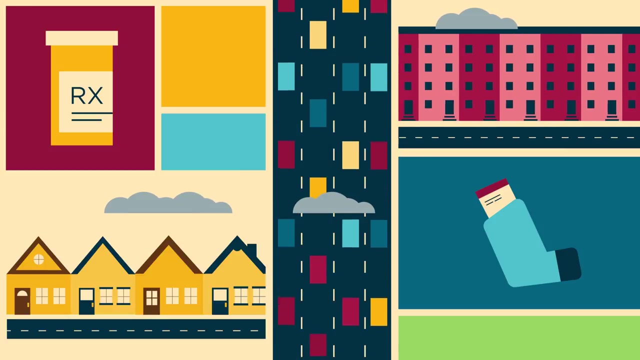 residents of all races are less upwardly mobile. And finally, despite being created to protect public health, zoning often pushes multifamily buildings closer to highways in areas with higher concentrations of air pollutants. As a result, low-income people and people of color are more likely to live in places. 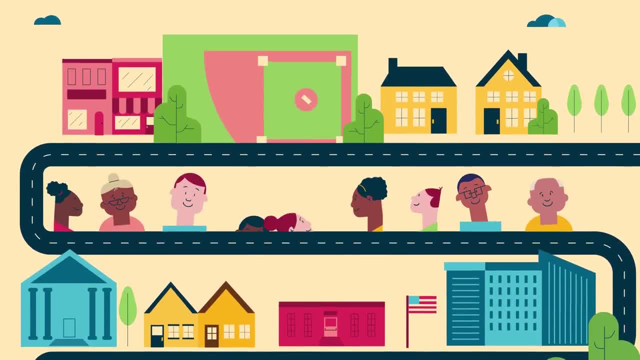 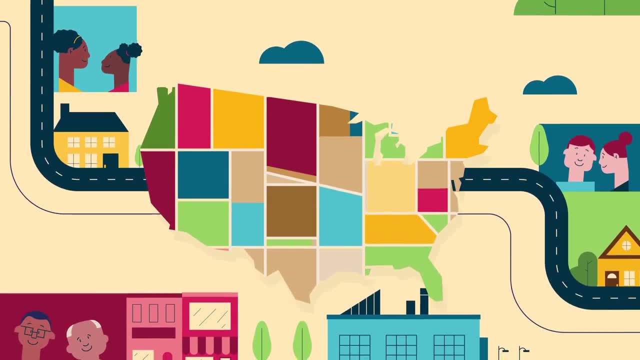 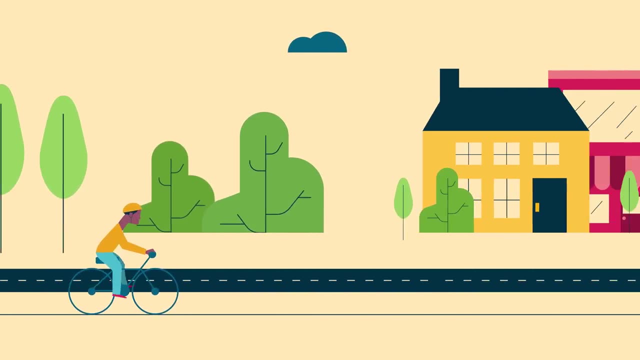 that could make them sick. It doesn't have to be this way. When done thoughtfully, zoning can connect people and places, not divide us. Communities across the United States are beginning to re-examine the role of zoning and change the restrictive zoning rules, opening neighborhoods to multi-family. 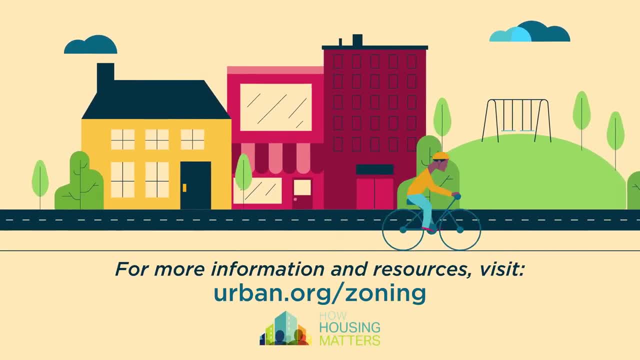 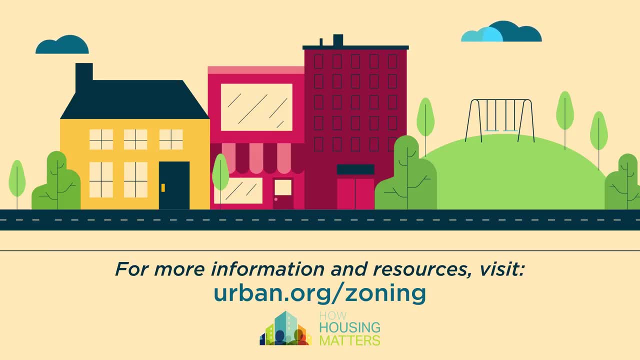 housing, walkable densities and more. For more information and resources and to find out what other communities are doing to improve their zoning policies, go to urbanorg: slash zoning you. 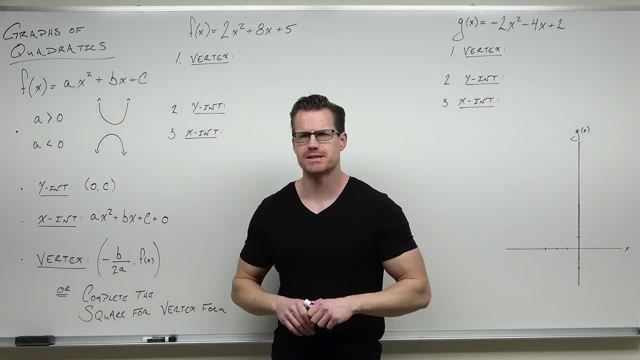 Hi, welcome to another video. In this video we have something very basic. We're going to talk about the properties and graphs of quadratic functions, how to kind of come up with this vertex form, versus maybe just graphing the vertex and x-intercepts and y-intercepts, that they work. 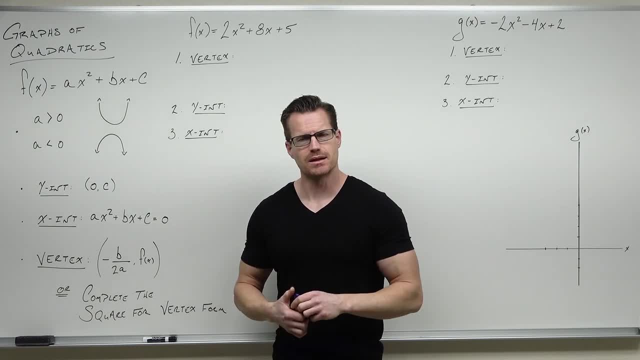 together just one time through, to make sure that you're seeing it. This is a little more advanced than like an intermediate algebra class, because none of these are going to be factorable for us very easily. So we need to find x-intercepts through quadratic formula, but basically just.